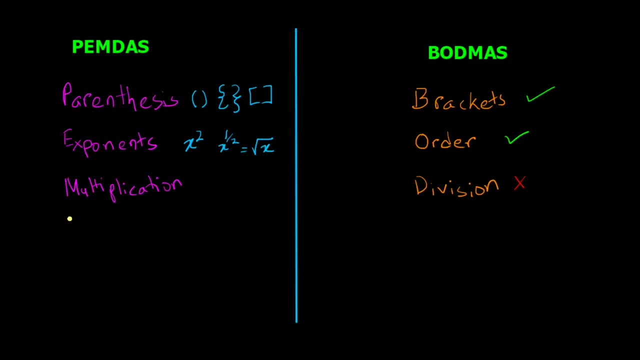 The letter looks different here as well, So it's D, which is division, And BODMAS is M, which is multiplication, And they're definitely not the same either. Okay, let's look at the next one. The next one is A and S, for both sides. 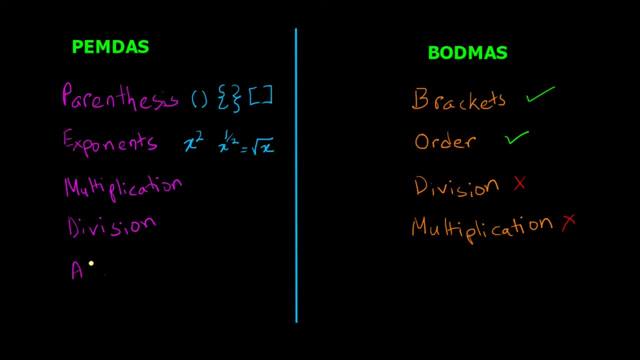 Looks the same by the letter. Let's see what they mean. This one is addition and subtraction, And over here it's Addition and subtraction. These two are definitely the same, So the problem over here mainly comes down to these two parts. 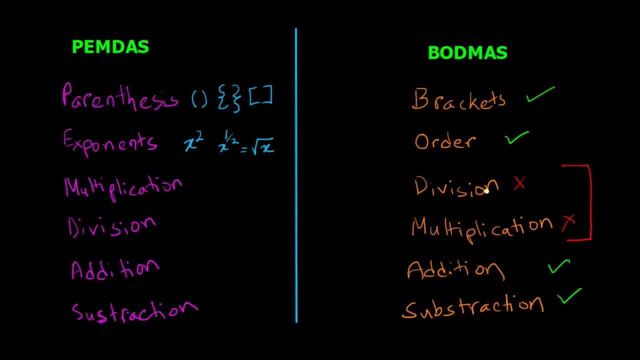 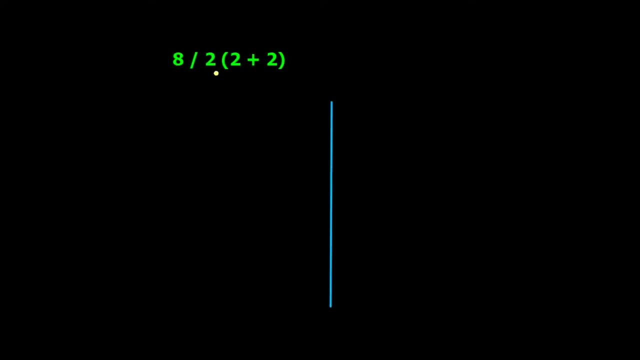 One is saying multiplication first, The other one is saying division first. So, in order to demystify this, let's look at an example. Let's look at this example right here. So this is the equation that took social media by storm. 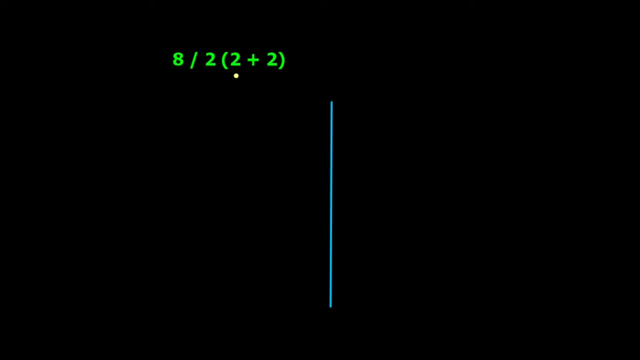 And a lot of people were arguing what the answer for this should be a few years back in different social medias. So let's try to solve this and see how PEM does and BODMAS answers this question. So for either one, brackets should be first. 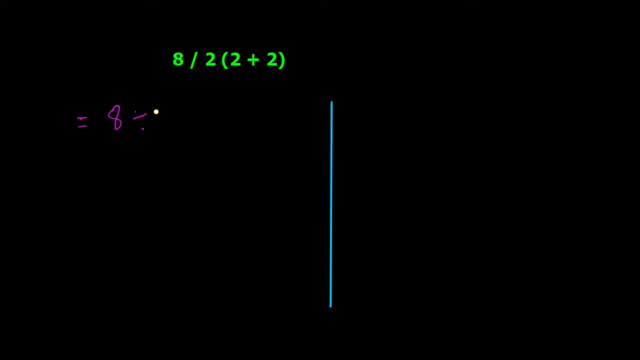 So I'll just write that down. 8 divide. I'll just try to divide like this: 8 divided by 2.. 2 plus 2 is 4.. Write it down. And then 8 divided by 2.. 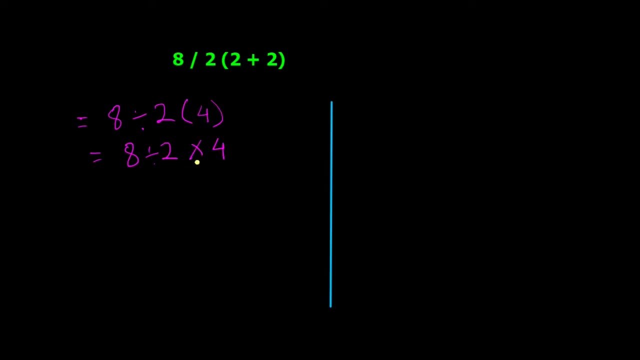 And then this bracket is basically multiplied. right. I'll do This is the PEMDAS. I'll do the BODMAS one right now. So the first step should be same And the second step also is same till now. So everything looks same till now. 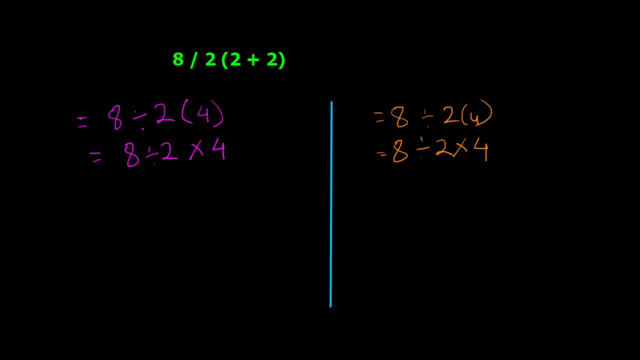 But for PEMDAS multiplication came first right. So the answer should be, If we follow the order there, 8 divided by 2. Not 2. 8. Multiplication is first, So 8., And then it should be 1.. 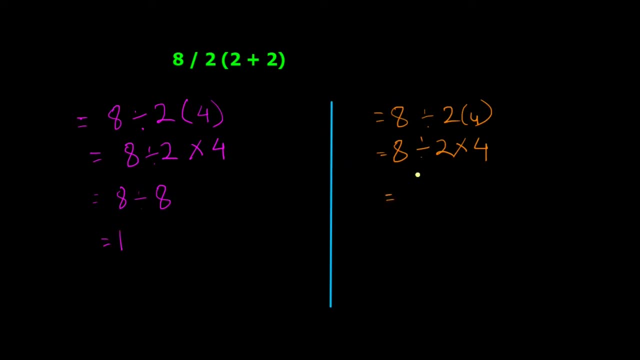 And for BODMAS the division should be. It comes Division comes first in the acronym. So 4 times 4.. And 4 times 4 is 16. 16. So they're definitely not the same. And something is happening. 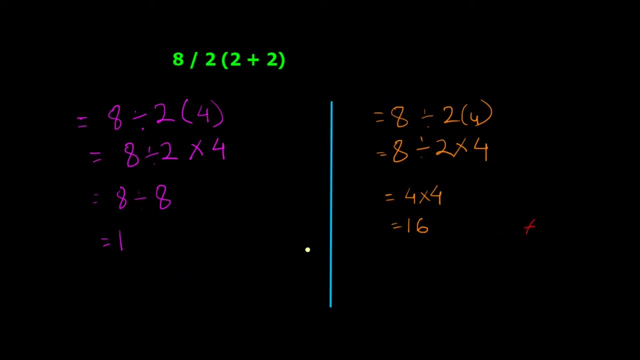 These are not the same. Something is happening over here. So in mathematics, if we don't consider these acronyms, what the main way to do this equation is? by using different orders, like levels, when it should be done first. So let's look at the example which should be done first. 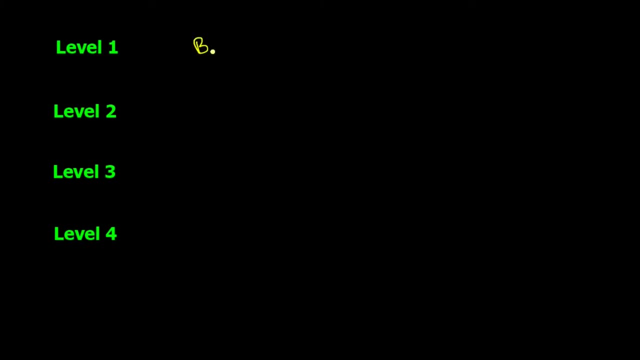 For either case, I think we saw brackets should be the first one And then exponents. I'm using brackets from BODMAS and exponents from PAMDAS just to keep both of them in there, Okay, So anyways, the level 3.. 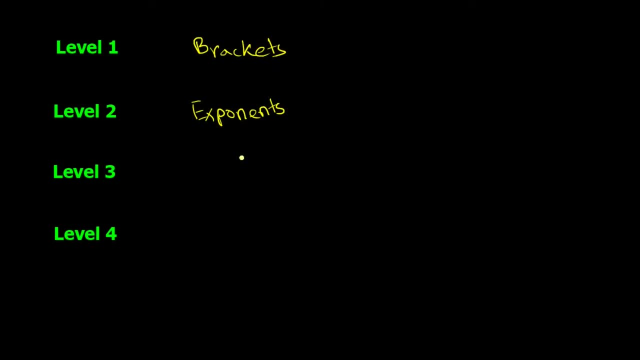 So brackets should be done first and then exponents, Both of them, and beyond that, The level 3 should be multiplication, Multiplication, Multiplication And Division. So they're together, They're on the same level, And level 4 should be addition. 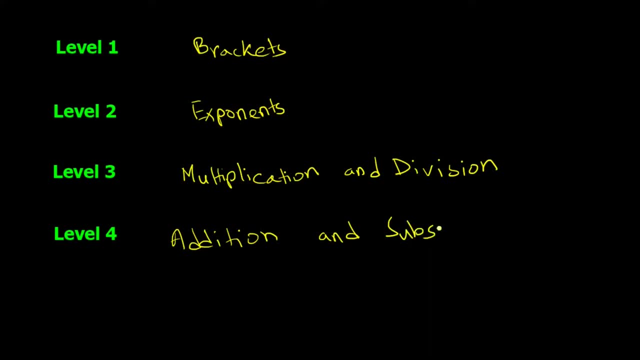 And Subtraction. They are on the same level. So multiplication and division is on the same level. Addition and subtraction is on the same level. What is the difference? Well, let's look at addition and subtraction first. Let's see. 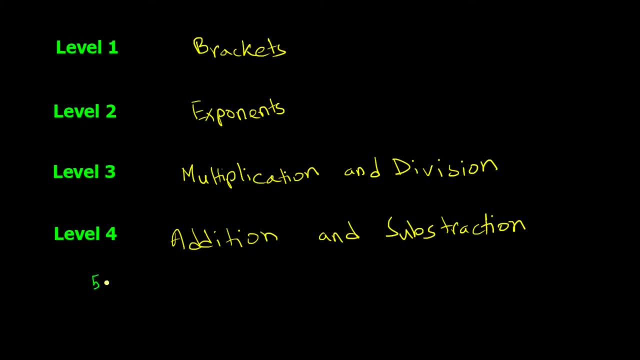 Let's see if they actually matter. So suppose we have 5 plus 5 minus 2.. So if I do addition first, what do I get? 10 and minus 2, which is 8.. Now let's do the same thing. 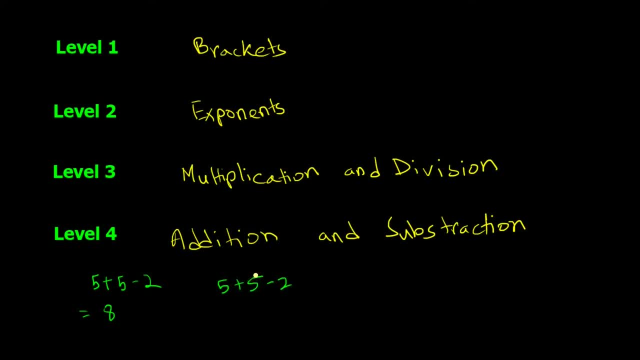 Well, let's do subtraction first: 5 minus 2. That's 3. And this is 3.. And 5 plus 3 is 8.. Let's do another one: 50 plus 2.. 50 plus 10 minus 20.. 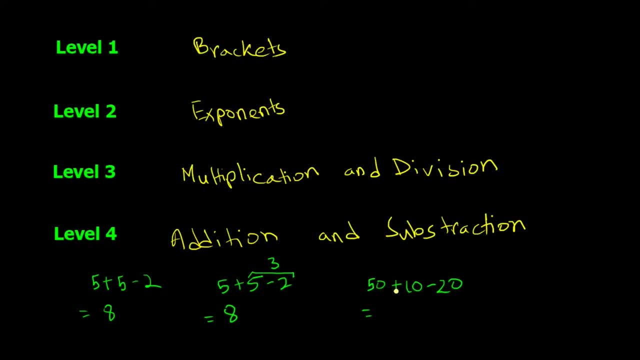 So let's do plus first: 50 plus 10 is 60.. 60 minus 20 is 40.. And then let's do again: 50 plus 10 minus 20.. Let's do subtraction first: 20 minus 10 is negative 10.. 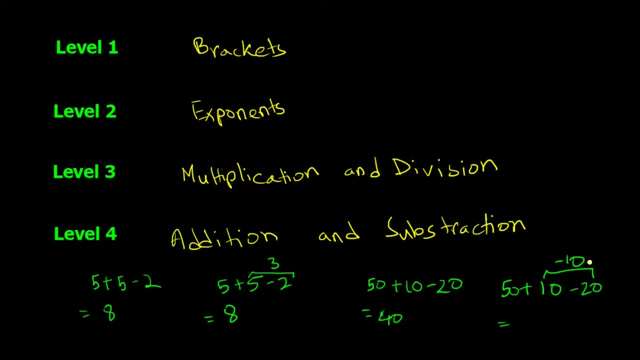 And 50 minus negative. 10 is 50 minus 10.. Positive and negative becomes negative. 50 minus 10 is 40 as well. So for addition and subtraction they are on the same level, But it doesn't matter which one you do first. 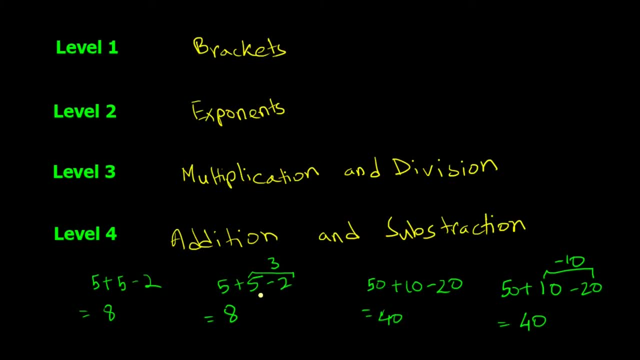 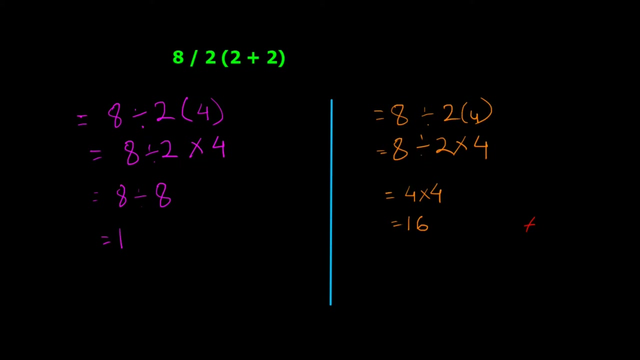 You can do addition first or subtraction first, The answer will be the same. But for like multiplication and division, as we have seen in this one, it really doesn't matter if we do division first or multiplication first, Right. However, the rule when you come across this equation like this is: 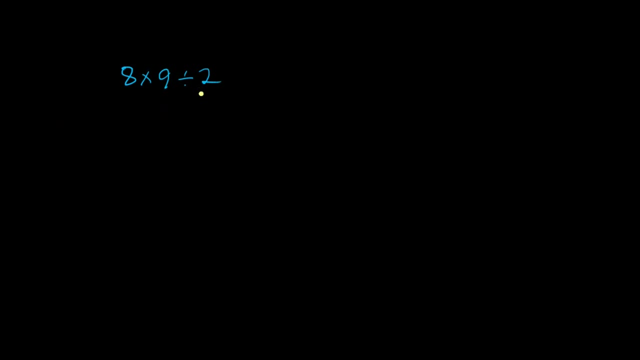 suppose we have 8 times 2 minus divided by 2.. The rule for this is you go from the left hand side. So whenever you have like multiplication and division on the same level, like on the same equation, you go from the left hand side. 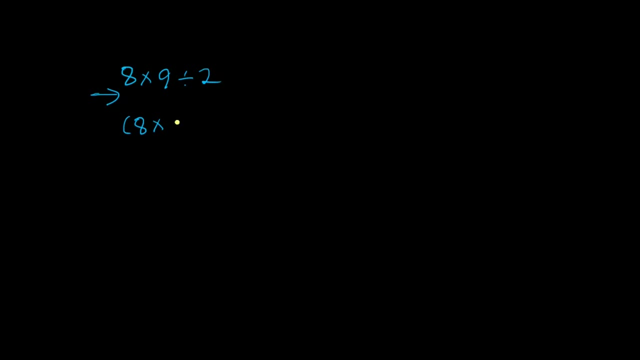 So it should be 8 times 9 divided by 2.. Similarly, if you have something like this: 8 divided by 9 times 2, you should go from the left hand side. So the first step should be 8 divided by 9.. 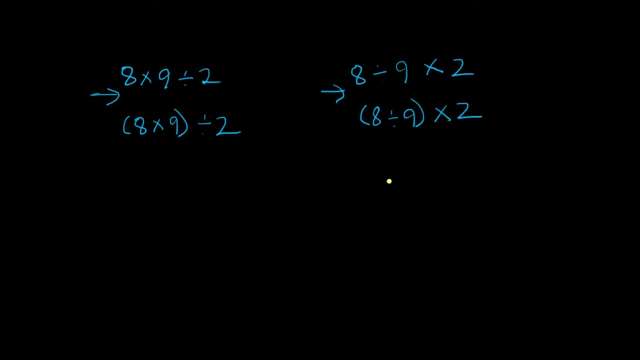 And then you multiply by 2.. In reality, there should not be any case where you get an equation like this, because it's a very ambiguous way of writing equations. Usually they should like specify with brackets beforehand, Then they should be done first. 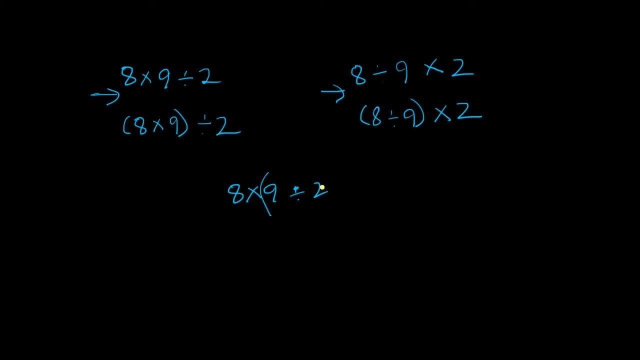 Or They should be done first using brackets. That's the way the equation should be written. But, however, for this specific case that we've seen the equation, the answer should be: We have seen up to this point. They are both the same.